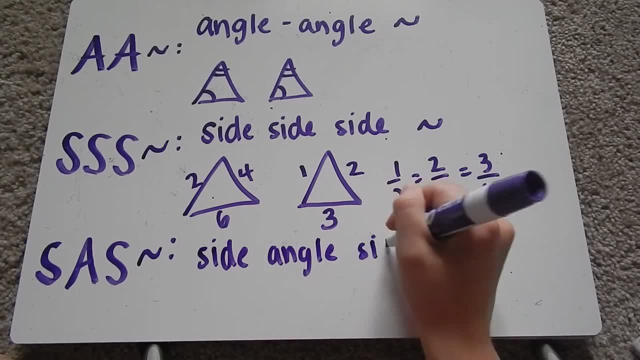 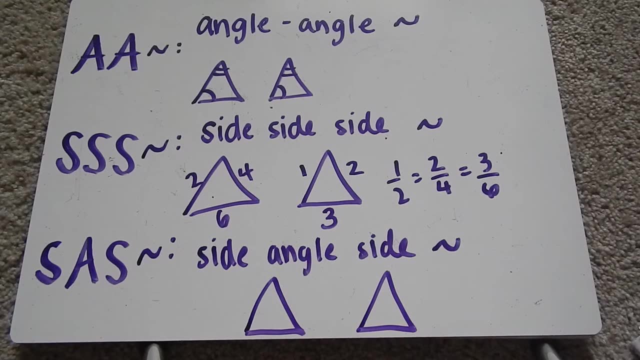 Side angle side similarity. So let me draw my triangles here. Notice how the angle is in the middle of the sides, which means wherever your angle, your angle has to be congruent. wherever your angle is, you have to look at the sides that meet to form the angle. 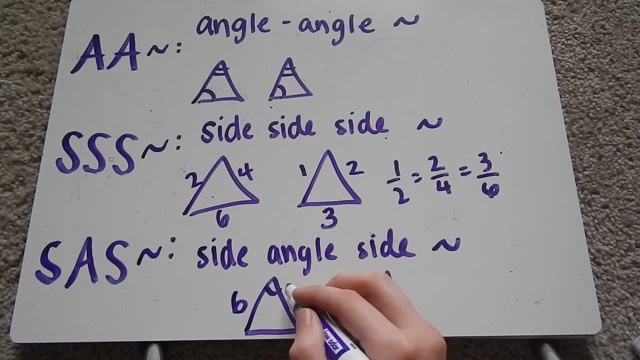 So if this side was 6 and this was 6, and this side was 10,, this side would also have to be 10.. They have to be proportionate. They don't have to. these sides don't have to be equal, but they do need to be proportionate. 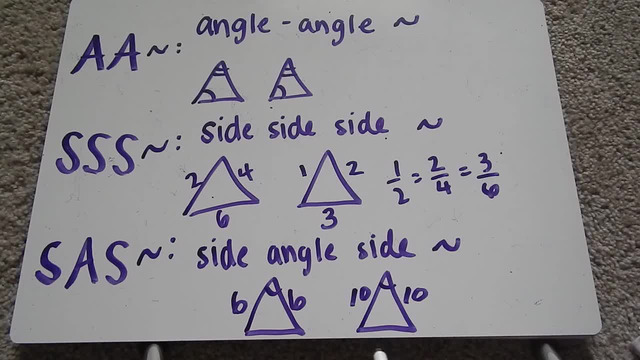 If you had, say, this side and this side were proportionate, that would not be side angle side, because the two sides have to include the angle. The angle has to be in the middle of the two sides, So this would be congruent. 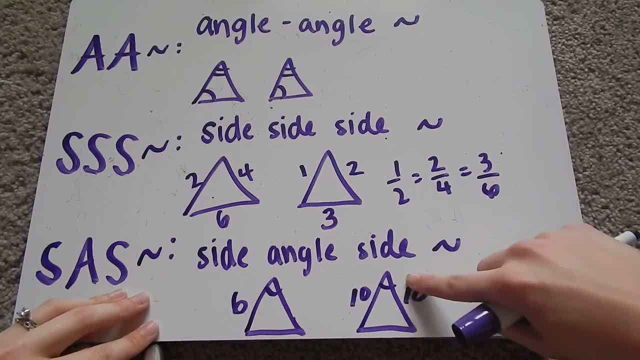 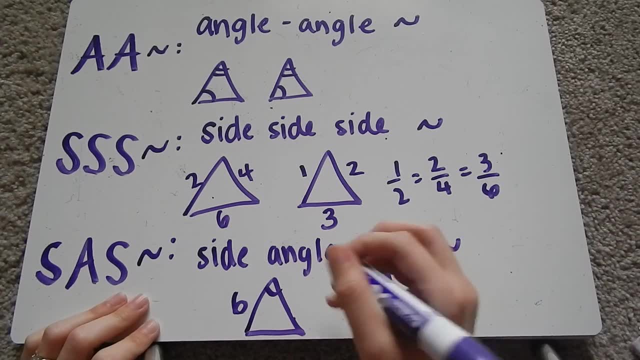 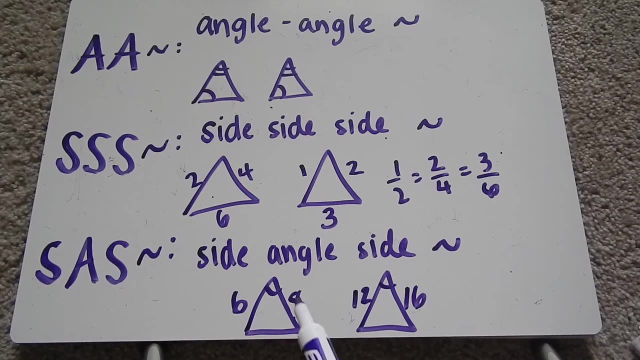 And this might be confusing, so let me change the numbers a little bit. If that was 6,, this is 12, and this is 8, that's 16,. those sides are proportionate, because I'm just multiplying by 2 to each one. 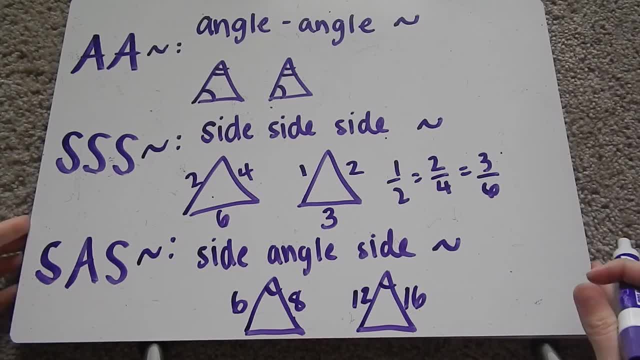 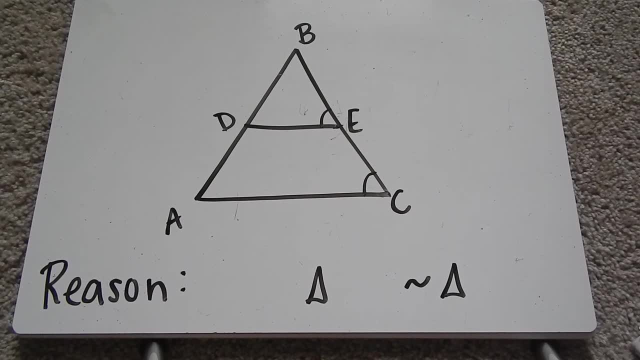 Angles are congruent. that's side angle, side similarity. Let's get started on some examples. We're going to determine if they're similar. If they are, we'll give them the reason And then we'll try to determine the corresponding parts of the triangle by naming it. 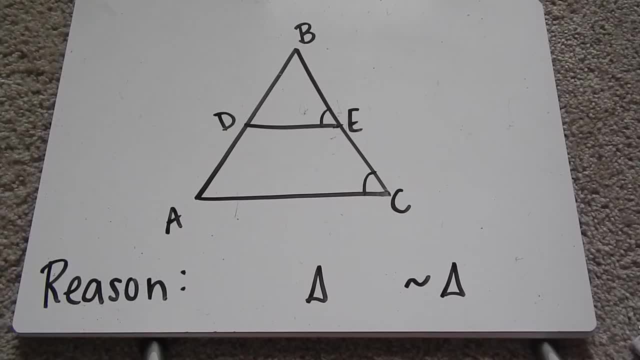 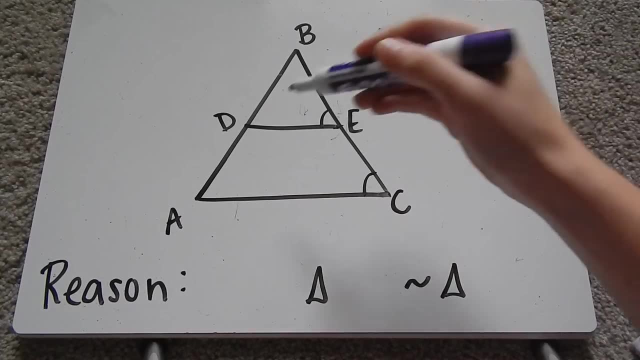 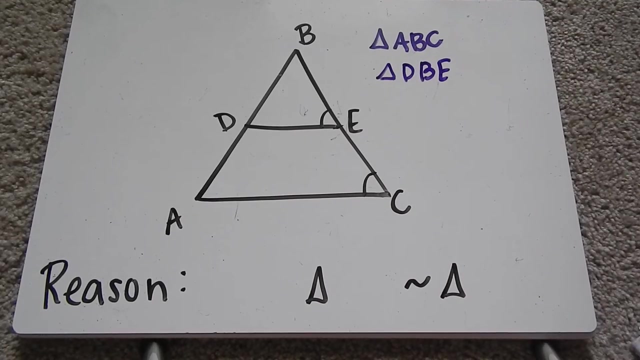 So if we look at our first example, let's look at the triangles that we have. We have this big triangle ABC, So I'm going to call triangle ABC. We also have this little triangle which is triangle DBE. I'm not naming that in any particular order. 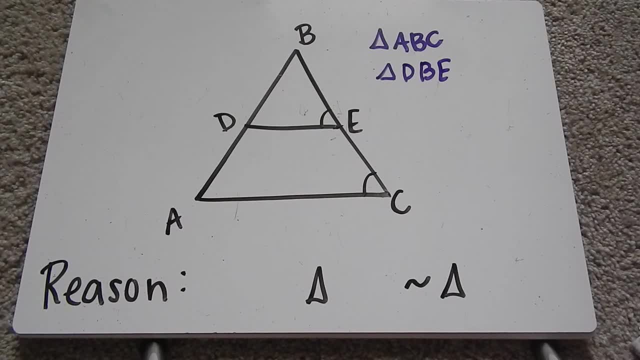 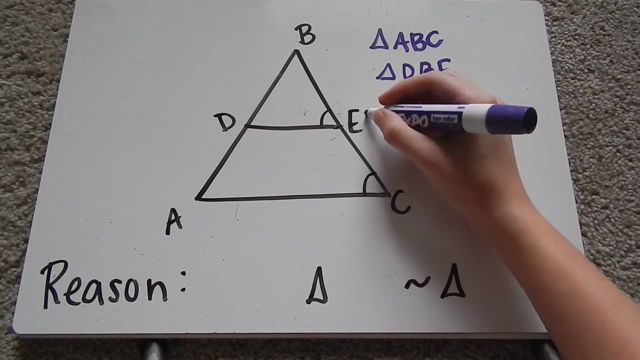 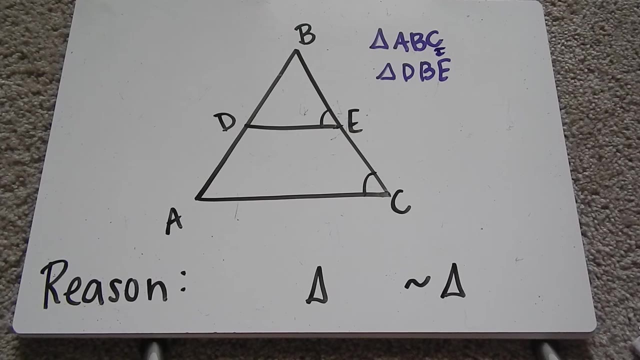 I'm just going by what I see. Now let's determine if these are similar. First of all, we're given one angle is similar, So E and C are congruent. Since E and C are congruent, if we have another angle that's congruent, we could use angle-angle. 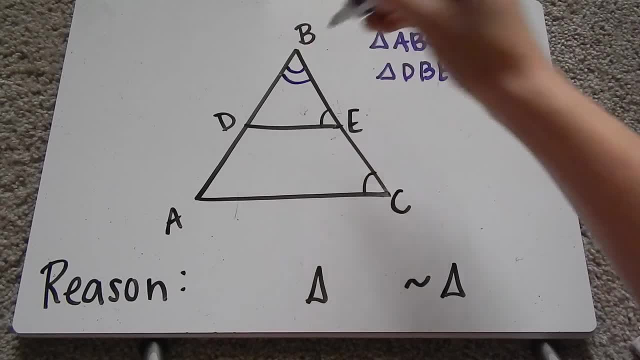 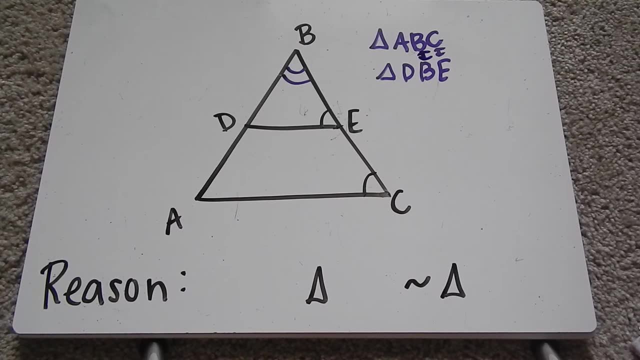 Well, if you notice this, angle B here is equal to itself. Both triangles use angle B. Angle B equals angle B. So we have similarity by angle-angle similarity, And actually how I wrote them here is how they're going to be written down here. 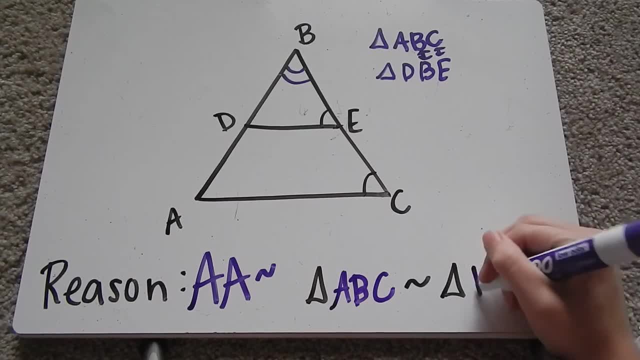 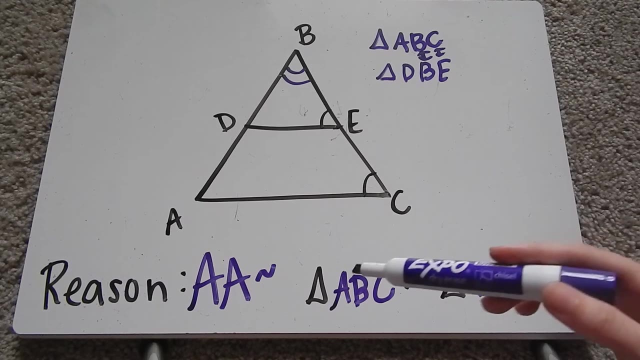 Triangle ABC is congruent to DBE. We know that because E and C are corresponding, so they have to be in the same place. B and B are corresponding, so they have to be in the same place as well. Okay, And so A and D would end up being at the front of how I wrote it here. 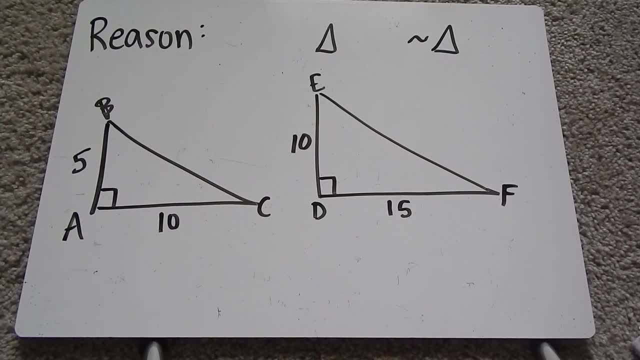 Moving on to our next example. Okay, again, we're going to do the same thing: figure out if they're similar, give a reason and then name them with corresponding parts. Now I see, here I have an angle. They're equal. 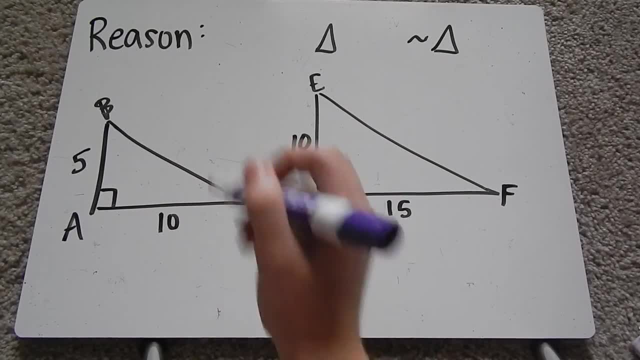 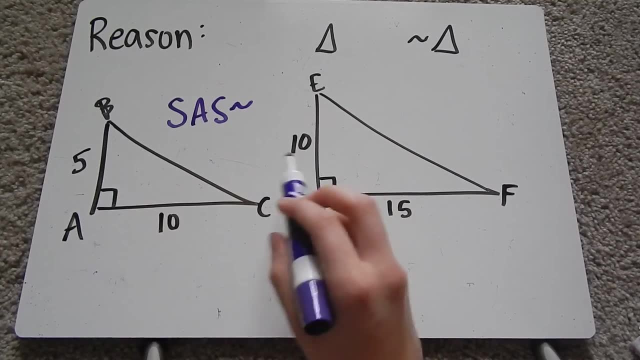 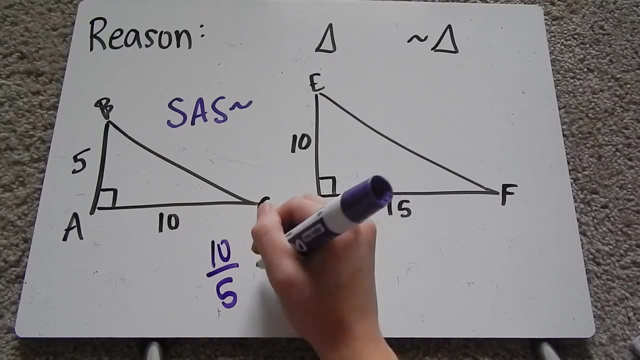 That's good And I have sides, So this could be a side angle, Okay, Angle side similarity. But we have to determine if these proportions are equal. So for this triangle to this one, I have 10 over 5. Okay. 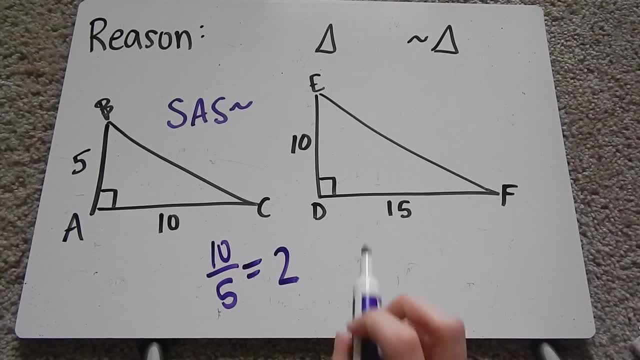 That if I reduce it equals 2.. So if I take side DF to AC, 15 over 10, that also needs to equal 2 for this to be, for these to be similar triangles. Well, 15 over 10 is actually 1.5. 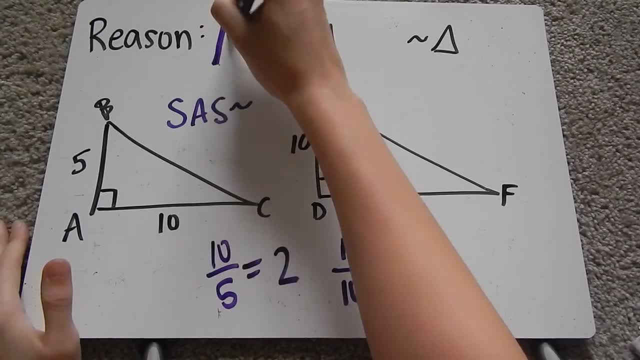 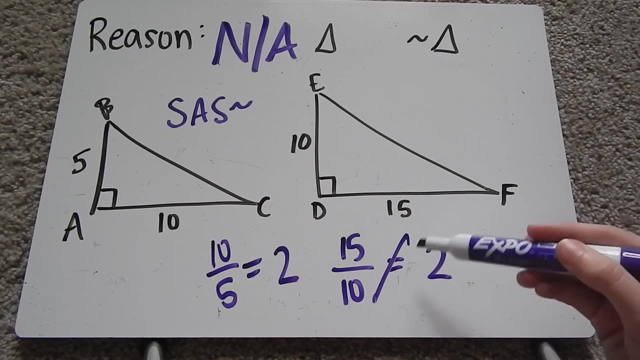 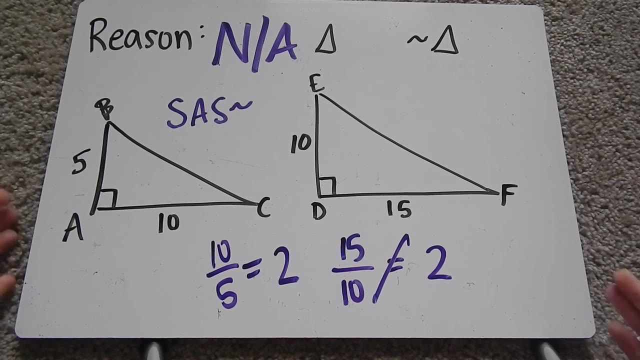 So that is not equal, which means these are not similar triangles. If this proportion happened to equal 20, or, sorry, 2,, then that would give me side angle, side similarity, But it doesn't Okay, so let's move on to our last example here. 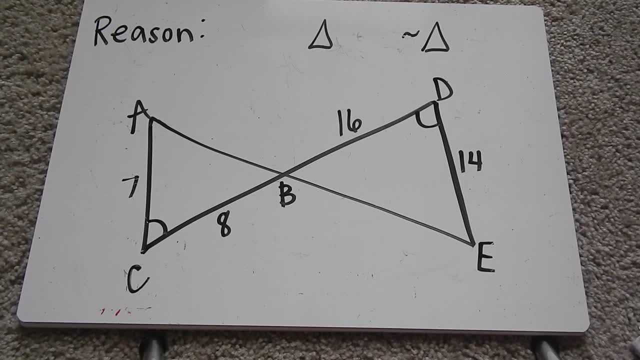 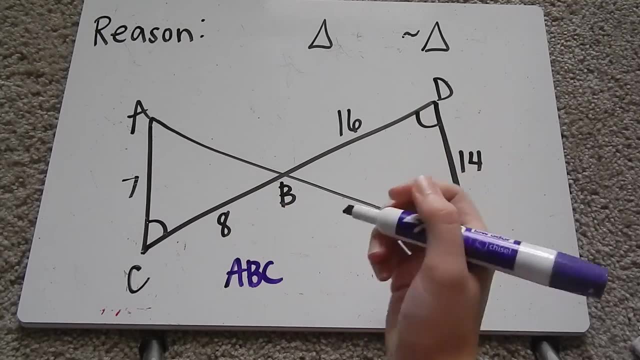 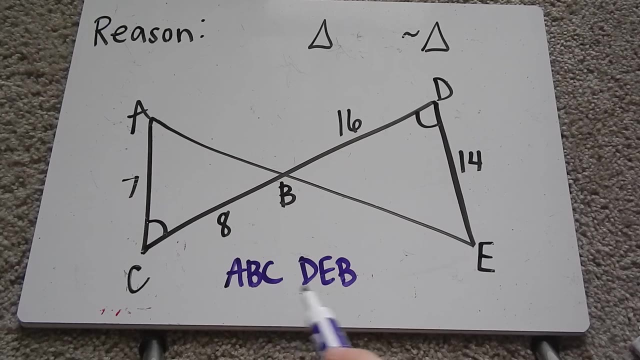 Okay, So again, let's talk about our triangles here. So I have a triangle ABC and I have this triangle DEB. We don't know any order yet, but we know these are our triangle names. Now I see I have C, and D are corresponding.